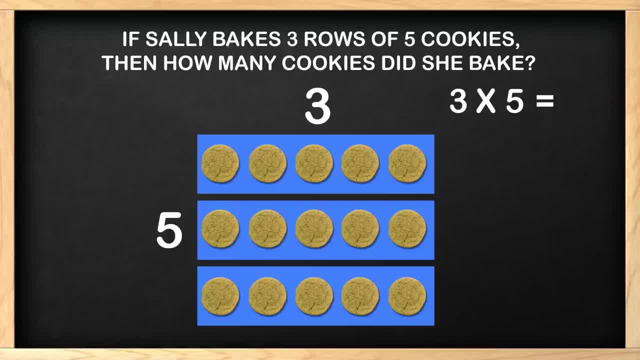 times five equals blank or what we do not know. We can now solve the problem in a couple of ways. We can count the cookies. There are one, two, three, four, five, six, seven, eight, nine, ten, eleven, twelve, thirteen, fourteen, fifteen. She baked fifteen cookies in all. 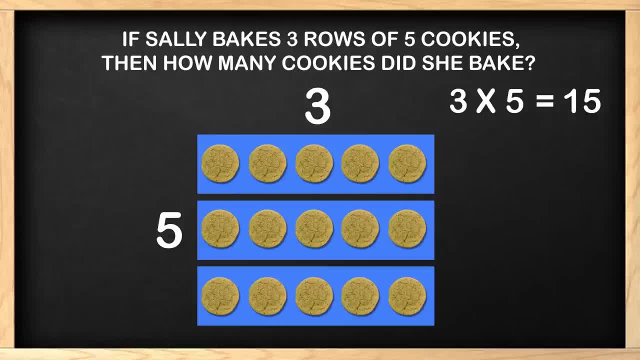 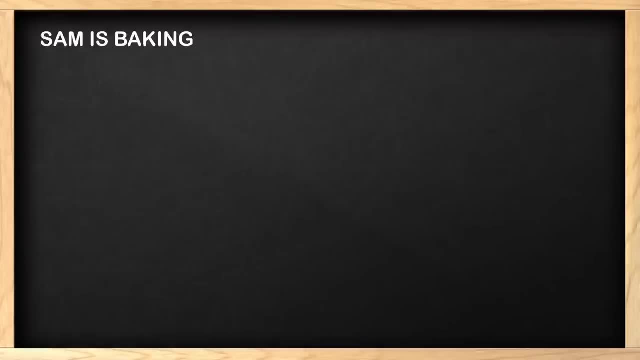 Instead of counting each cookie, we could also use our multiplication skills to know that three times five equals fifteen. Awesome, Let's look at another problem before I eat all these cookies: Robot. The new problem says Sam is baking twelve cookies. He puts. 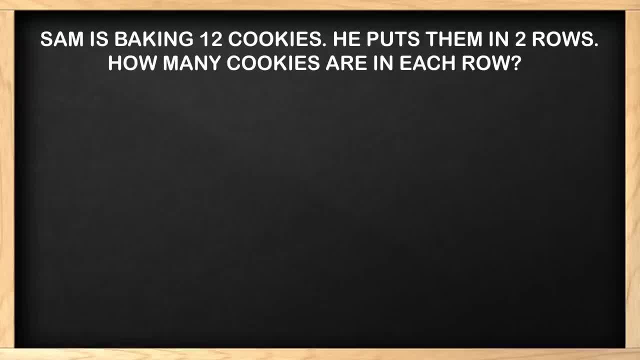 them in two rows? How many cookies are in each row? Before we jump in, let's not focus on if we are dividing or multiplying. We just want to first draw the problem. As you might have heard, the cookies got eaten from the first problem. Thanks, Mr Robot. We don't need the cookies to draw this. 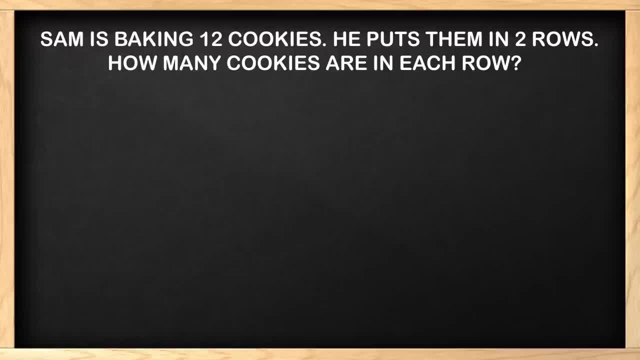 though We can just use tally marks. We know there are twelve cookies in all, and they are divided into two rows, so let's draw the two rows where the tally marks go. We are now going to put a tally mark in each row as we count to twelve. 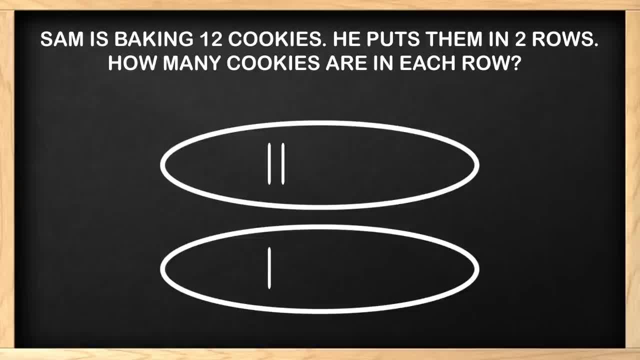 One, two, three, four, five, six, seven, eight, nine, ten, eleven, twelve. We have placed twelve tally marks in the two rows. How many are in each row? There are six tally marks. Great job, We solved the problem by just using the drawing. Let's write the equation that: 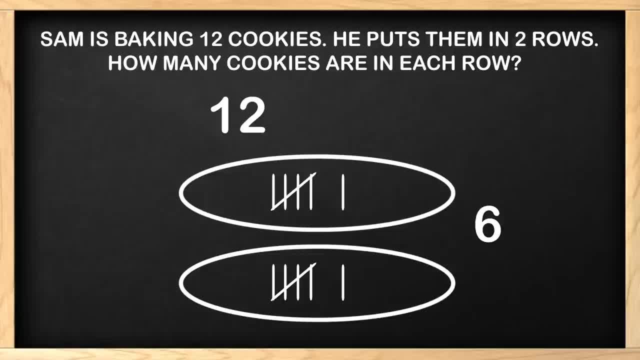 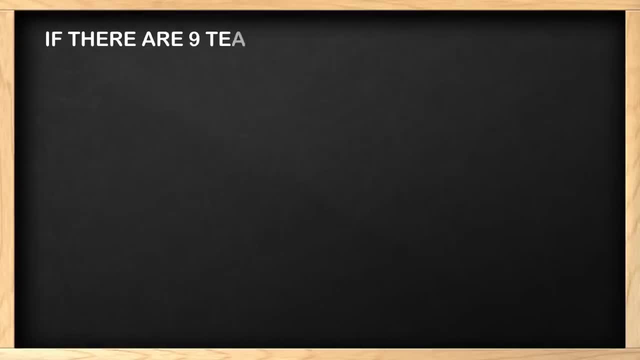 goes along with it. We started with 12 cookies and we essentially divided them into 2.. Our equation is: 12 cookies divided by 2 equals 6.. Great job, guys. That was amazing. The new problem says: if there are 9 teams with 9 players on each team, then how many? 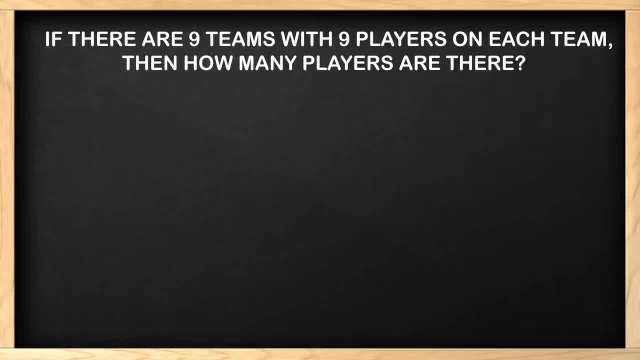 players are there. We could start by making tally marks to help us solve this problem. We have 9 teams and each team has 9 players. We basically have 9 groups and we'll put 9 tally marks in each box. Then we will count them all to see how many players there are. 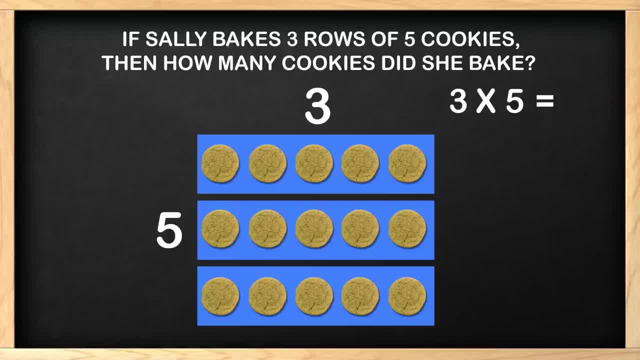 times five equals blank or what we do not know. We can now solve the problem in a couple of ways. We can count the cookies. There are one, two, three, four, five, six, seven, eight, nine, ten, eleven, twelve, thirteen, fourteen, fifteen. She baked fifteen cookies in all. 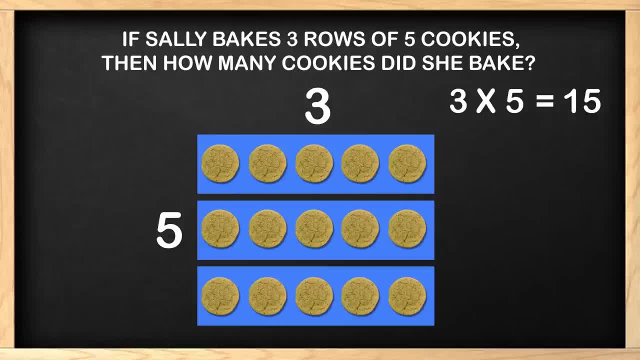 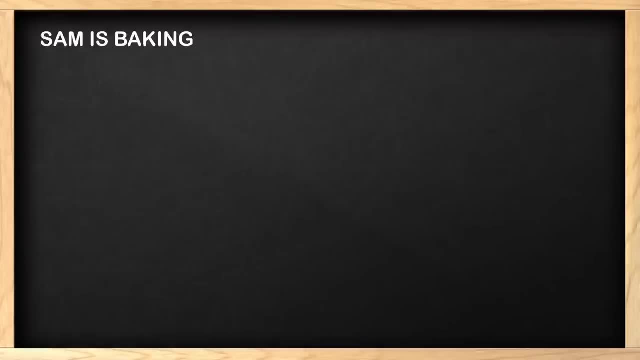 Instead of counting each cookie, we could also use our multiplication skills to know that three times five equals fifteen. Awesome, Let's look at another problem before I eat all these cookies: Robot. The new problem says Sam is baking twelve cookies. He puts. 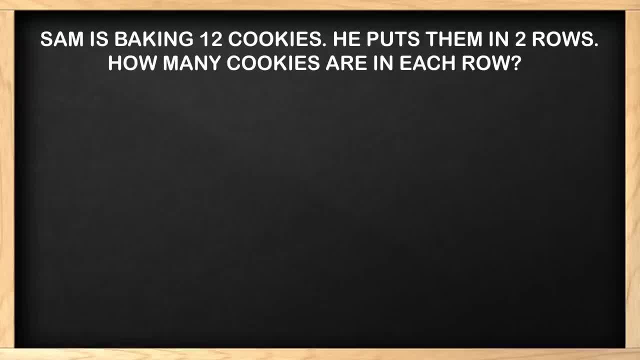 them in two rows? How many cookies are in each row? Before we jump in, let's not focus on if we are dividing or multiplying. We just want to first draw the problem. As you might have heard, the cookies got eaten from the first problem. Thanks, Mr Robot. We don't need the cookies to draw this. 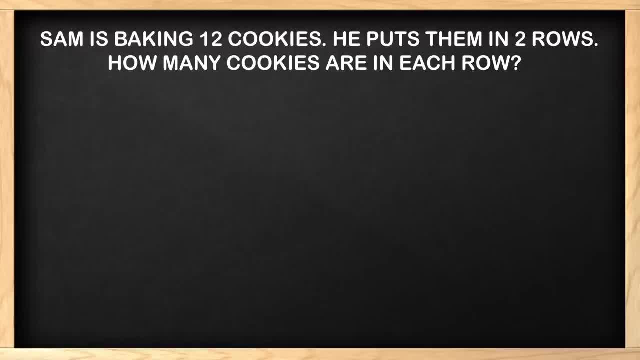 though We can just use tally marks. We know there are twelve cookies in all, and they are divided into two rows, so let's draw the two rows where the tally marks go. We are now going to put a tally mark in each row as we count to twelve. One, two, three, four, five, six, seven, eight. 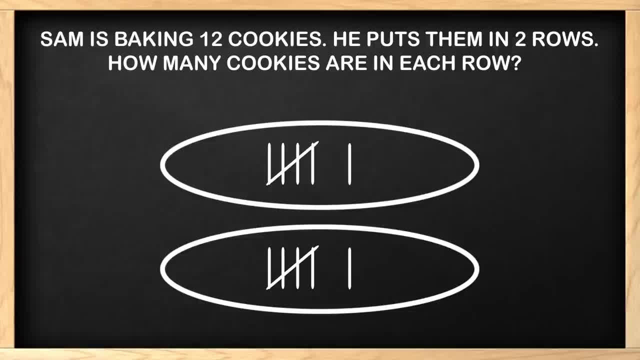 nine, ten, eleven, twelve. We have placed twelve tally marks in the two rows. How many are in each row? There are six tally marks. Great job, We solved the problem by just using the drawing. What was it actually like? It was good. Thank goodness, you learned someadi for that. How. 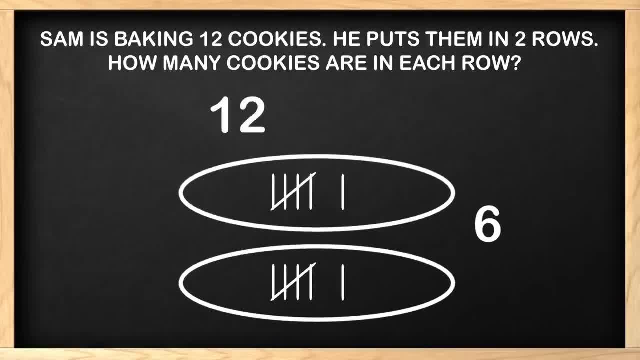 usual, Give your friends a hug. We don't have to waste too much time. I think you are getting an with it. We started with 12 cookies and we essentially divided them into 2.. Our equation is: 12 cookies divided by 2 equals 6.. Great job, guys. That was amazing. 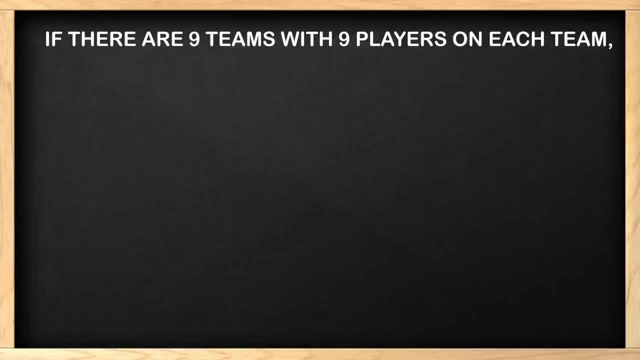 The new problem says: if there are 9 teams with 9 players on each team, then how many players are there? We could start by making tally marks to help us solve this problem. We have 9 teams and each team has 9 players. We basically have 9 groups and we'll put.